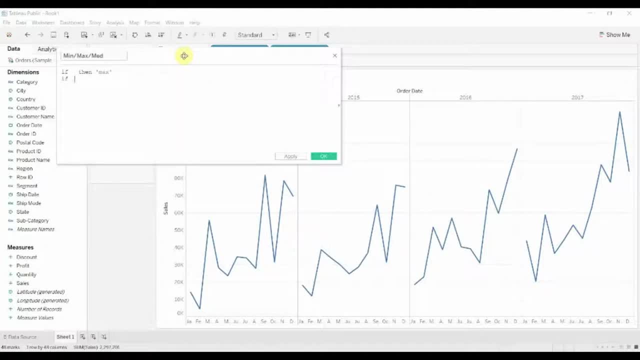 else, then it's the maximum. If else, if rather something else, then it's the minimum, Else it's medium. Now in here we want to say if the sum of sales is equal to the maximum of the sum of sales across some portion, And to do that we're going to use a table function. But instead of using a quick table function, we're actually going to create it by hand. And what the? 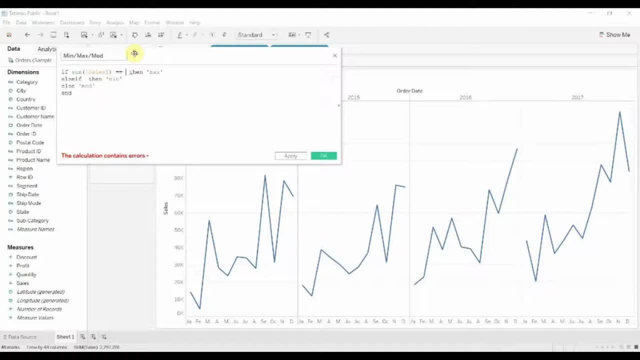 function that we want to use is window max. Window max will give us the highest value for whatever we tell it within a window that we can also specify. So we're going to say window max- sum of sales- Remember, we have to add an extra parentheses in there to make sure we're all balanced. And then for min, obviously we're going to do the same thing, But instead of using min, or sorry, instead of using max, we're going to be using the window min. 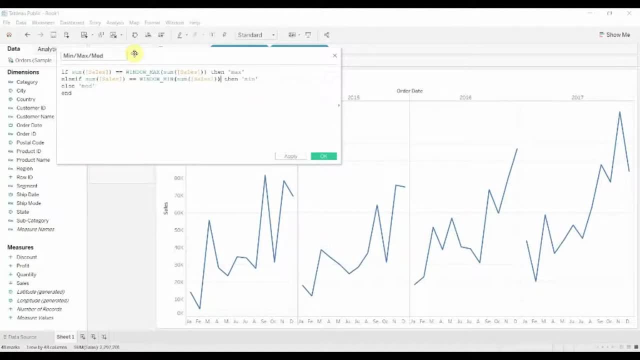 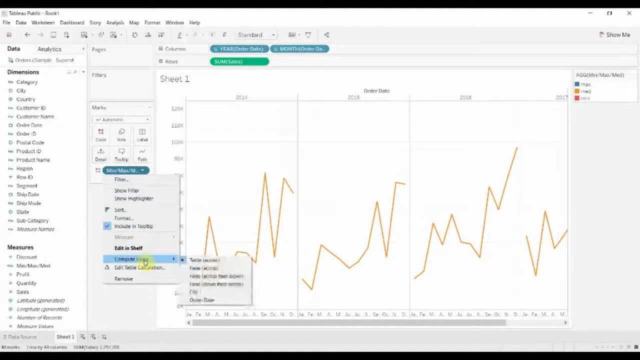 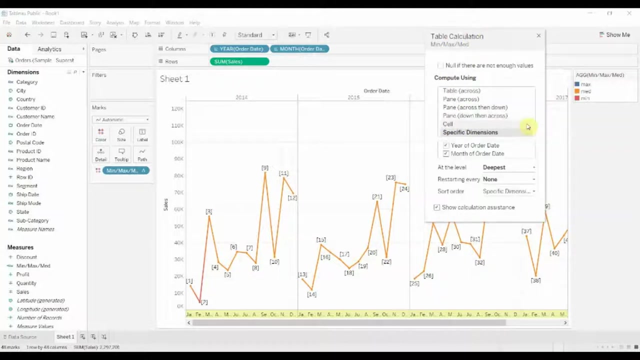 Add the parentheses in Perfect. Okay, So let's go ahead and drag this out to our color shelf. It's obviously not going to work first time out, because it never does, And then we have to specify within this how we want to use it. So we want to say specific dimensions. Right now we're only getting medium values, which is obviously not ideal. We just want to use 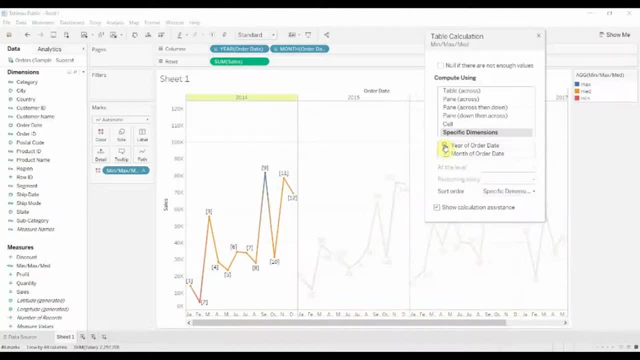 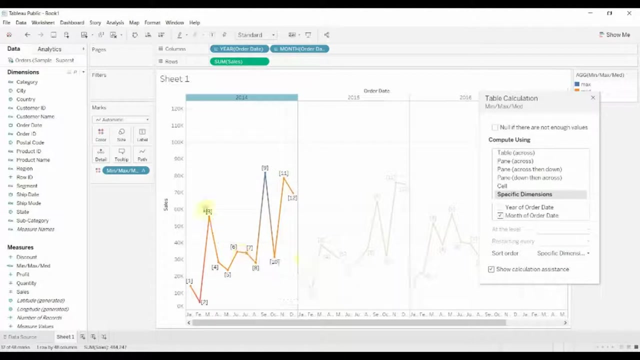 the month. And then now you can see- we're beginning to see- that we have the minimum month highlighted red, the maximum month highlighted blue, everything else highlighted orange, And that's the same, because we're only using the month, we're not using the year. So for every year it's just showing us the maximum and the minimum month. All right, awesome. Now, unfortunately, it looks a bit ugly, So